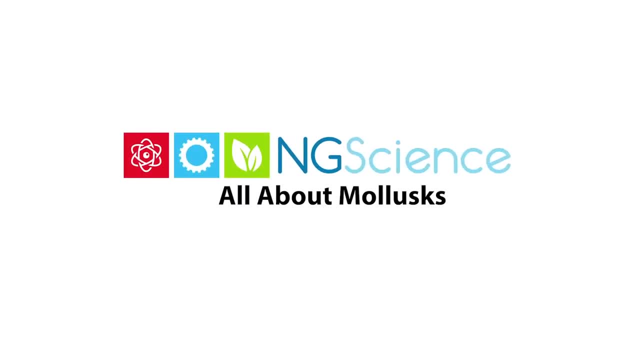 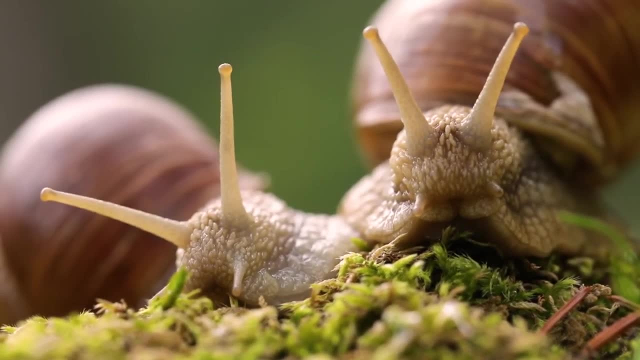 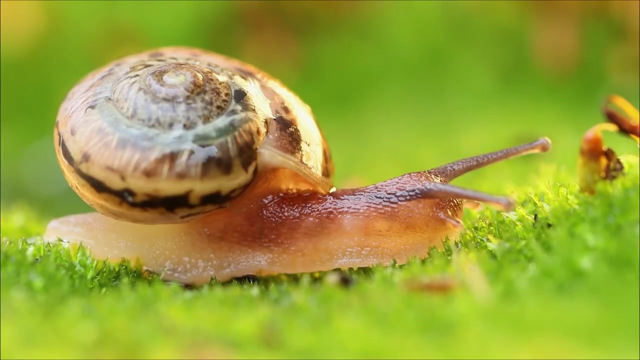 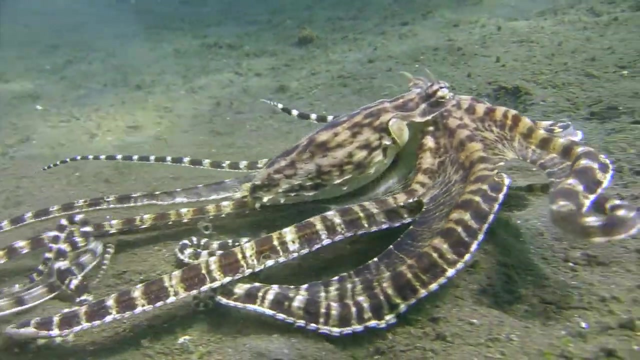 Mollusks are animals with soft bodies, sometimes with a hard outer covering called a mantle. Most mollusks live in the ocean, with some living on land or in fresh water. Scientists divide mollusks into three main groups: Gastropods, which include sea slugs, slugs and snails. 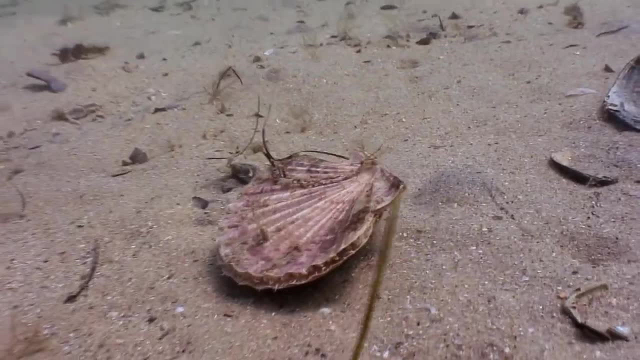 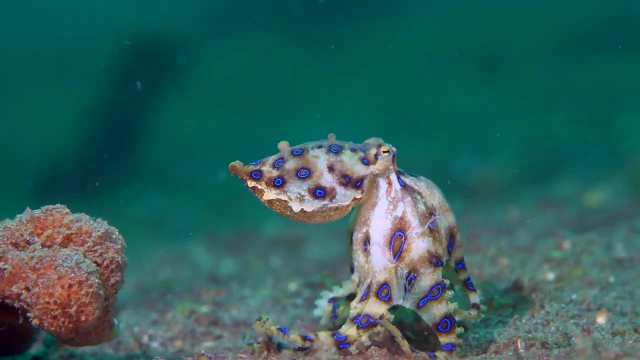 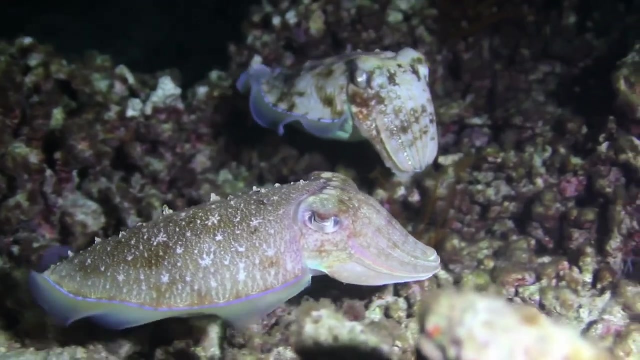 Bivalves, which include clams, scallops and mussels, And my favourite of all mollusks, cephalopods, which include octopi, squid and cuttlefish. The soft body of mollusks contains tissues and organs to carry out life processes. 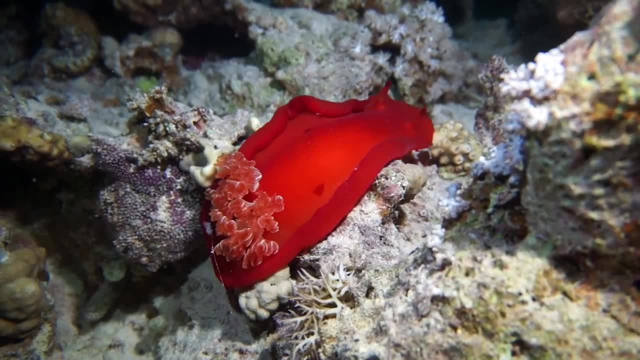 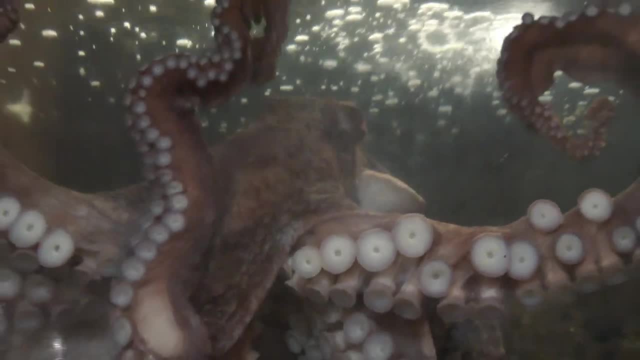 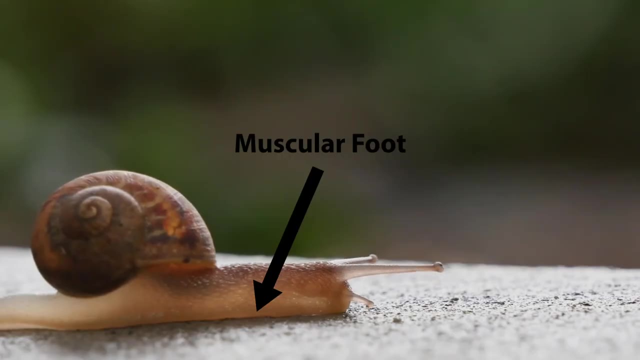 They have digestive, respiratory and circulatory systems. Most mollusks have a specialised mouth structure called a radula, which is a series of tiny teeth used for scraping food particles into the mouth. Mollusks also have a muscular organ called a foot, which is used to move about. 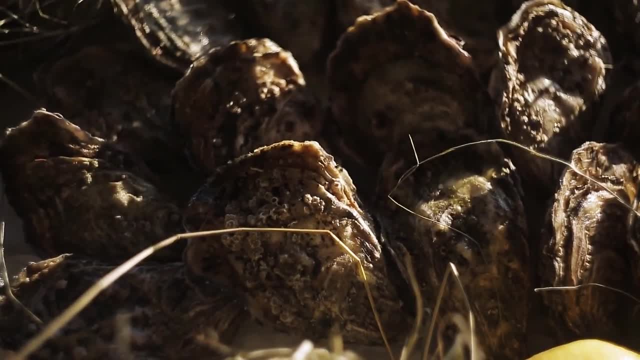 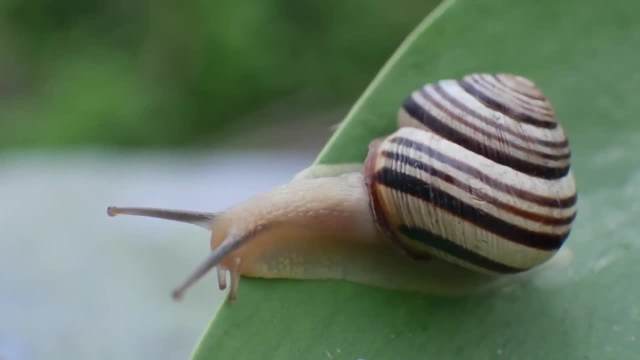 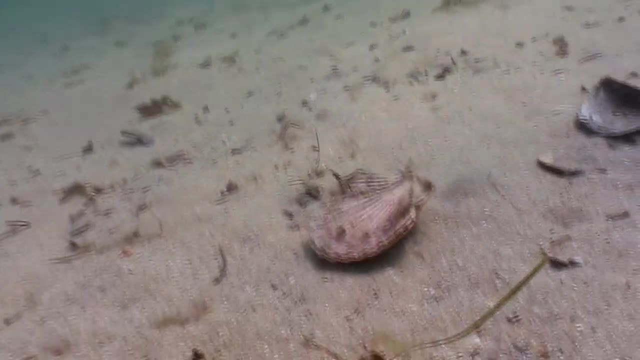 A common characteristic of mollusks is a mantle in the form of a shell. Snails and limpets are examples of mollusks with one shell. Clams and scallops have two shells which are hinged on one side. This allows the shell to open and close. 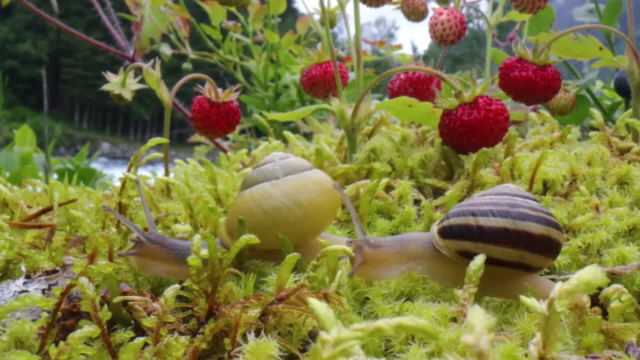 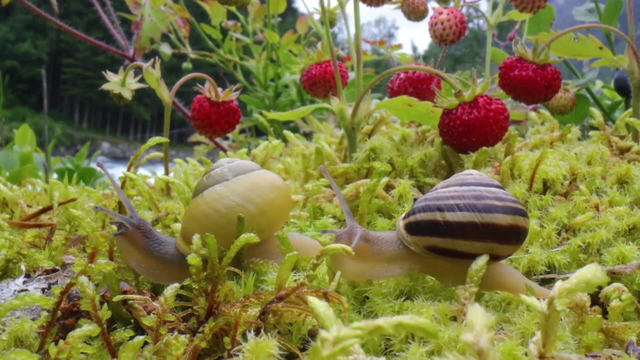 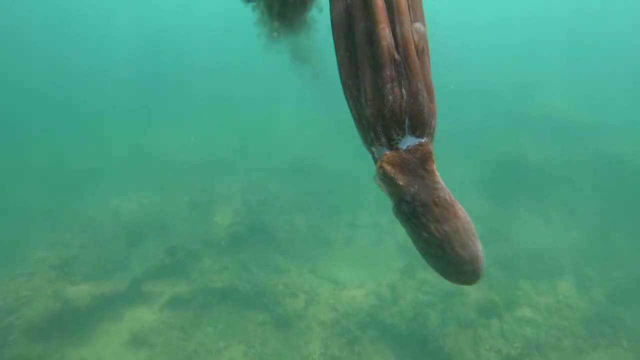 All mollusks have bilateral symmetry. All mollusks reproduce sexually, which involves the fertilisation of male and female sex cells. Cephalopods are thought to be the most intelligent of all invertebrates. Their large and well-developed brain makes them very efficient predators. 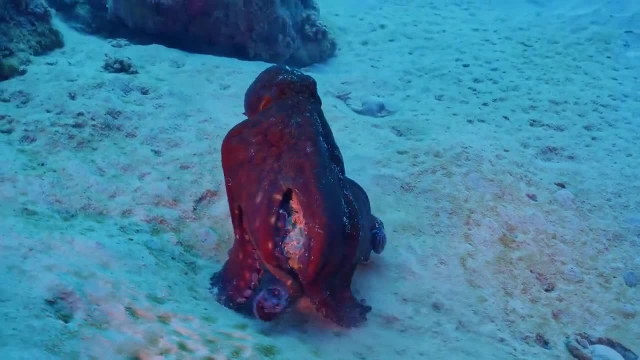 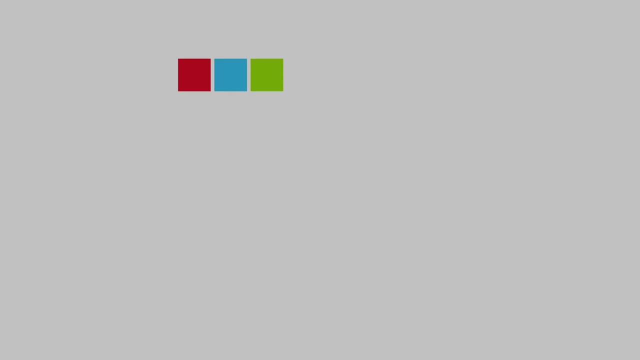 They are known to use tools and have demonstrated advanced learning and problem-solving abilities in laboratory environments. However, they have also been found to be weak, much more resilient. Therefore, it is important to know how they grew their body or teeth and what they do when they are out and about. and how they have a natural ability to produce this new trait of health. If you would like to learn more about mollusks, I have put up a video called a molly-bill in the video description.